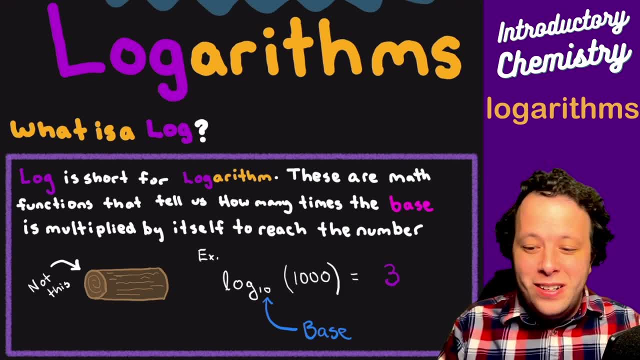 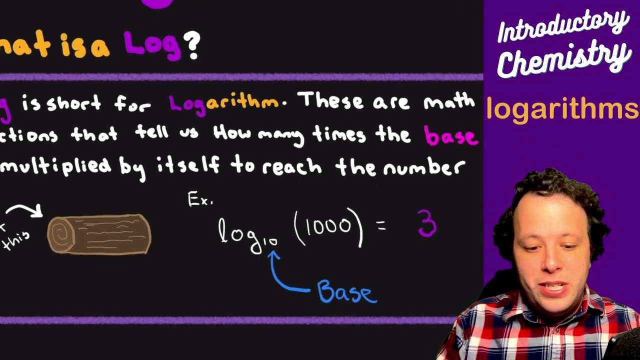 so log for short. we're not talking about the piece of wood here, but when it comes to logs or a logarithm is that these are math functions. And now with that function, what it does is it tells you how many times a base is multiplied by itself to reach that number. So what do I mean by that? to kind of make them make a little bit more sense. So most of the time in chemistry we're using a log 10 function. 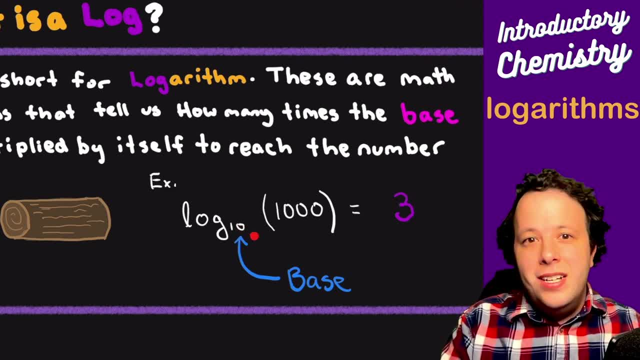 So this is referred to as the base. Now, in order to make this operation make sense, we have this 1000 number here. So we are going to use the log to take the function and we want to know how many times this 10 fit in this number. So if you think about that right, you do 10 times 10, that's 100 times 10 again and that is 1000.. It went into that 3 times 2 to see how many times the base fit. So the answer would be 3.. 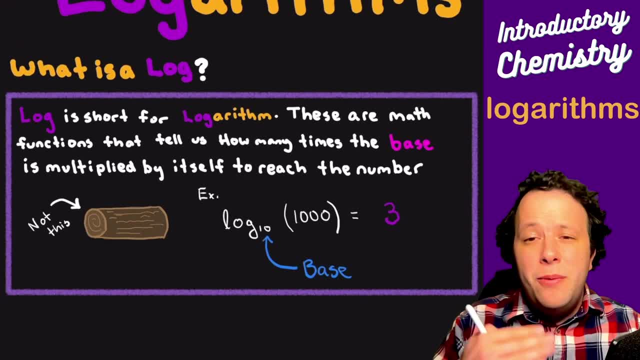 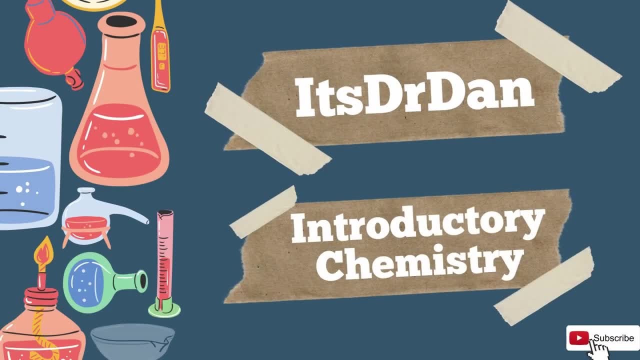 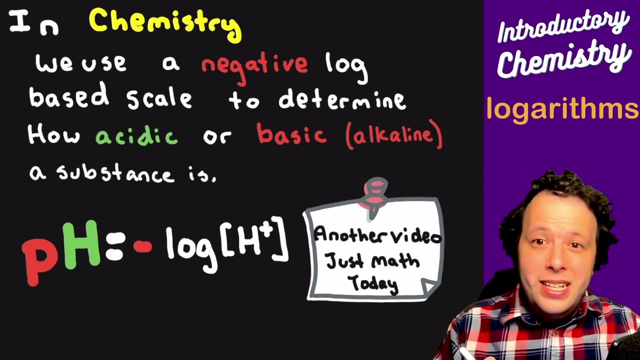 So that's kind of the idea here is that we're trying to figure out: well, can we make a simpler system? So what? how is that exactly used in chemistry? Let's take a look. In chemistry it's very common that we use scientific notation to denote different scales, And the general reason why we use that is because it helps simplify a lot of the numbers we use. 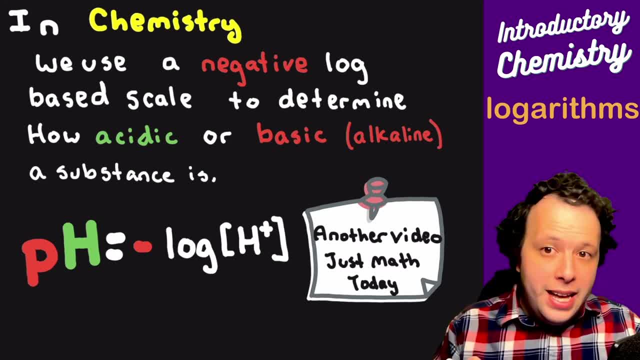 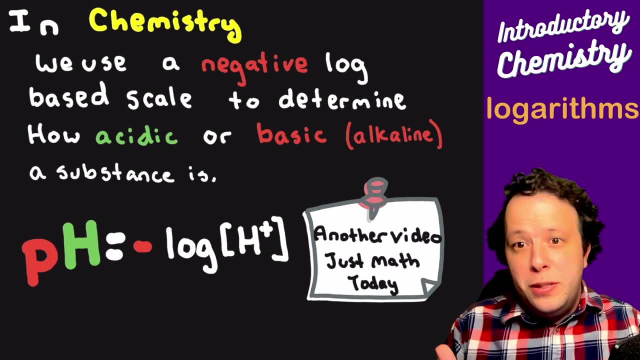 So one thing is that we commonly use a number Negative log base scale to determine how acidic or how basic a substance is, which is known as pH Right. You use pH in chemistry and biology and environmental science. You use it all the time. So with the pH, all it is is equals to the negative log and we're taking the function of the concentration of the acid. So what we do is we plug in the molarity of H plus into the log function. 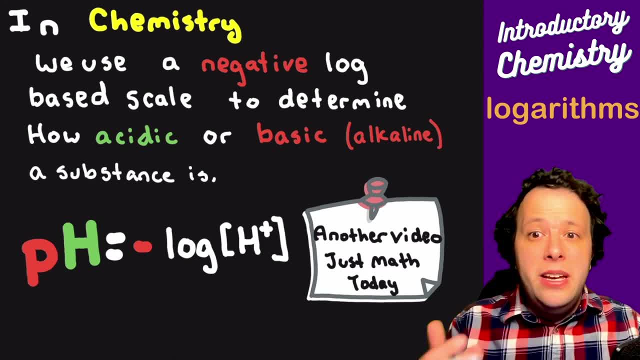 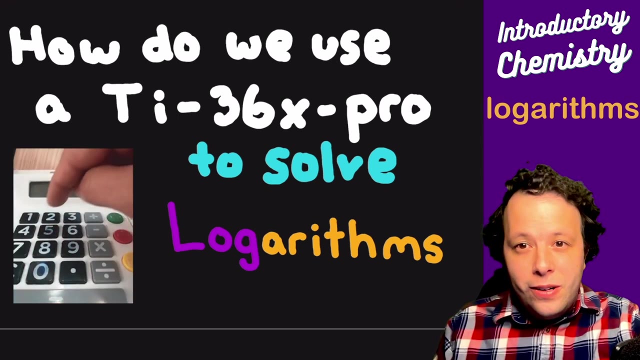 And we will get a pH, And we can do the same thing for POH as well. Now, the point of this video is not to talk about pH in the concepts behind it. That's another video which I would recommend referring to. But we are just going to look at the math and how to use your calculator to do log functions. Let's go into this a little bit farther: Which calculator you're used to. So we're going to be using a TI 36X Pro, So Texas Instrument Calculator. 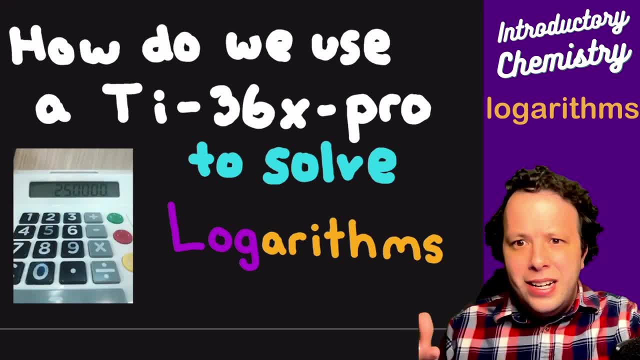 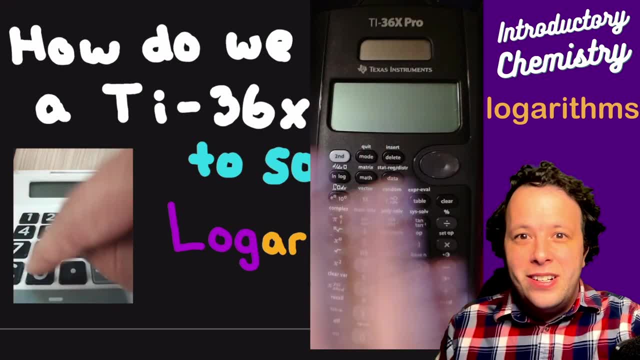 And also be giving tips and tricks on, like the TI-83 and the TI-88, which are other calculators which are very similar as well. So what we'll be doing is we'll be showing my calculator display here, So I'll be kind of. 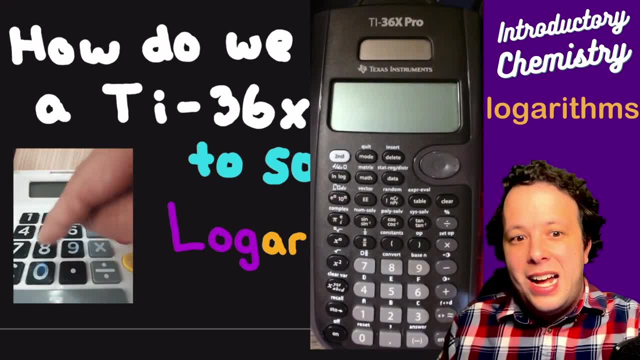 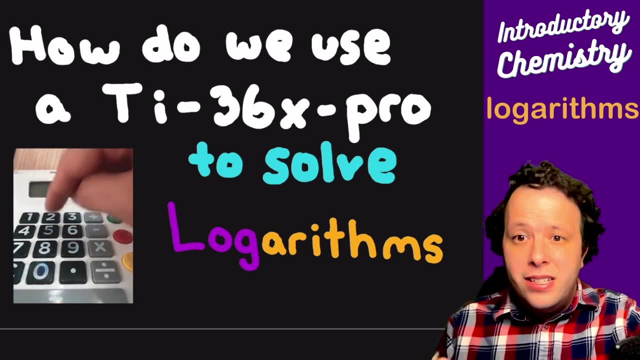 showing you the different buttons to hit. So that way you can get an idea of exactly what this guy looks like. So that way you can follow along with your calculator- And I would recommend trying to practice it along with me- So that way you can see: are you entering them in right? 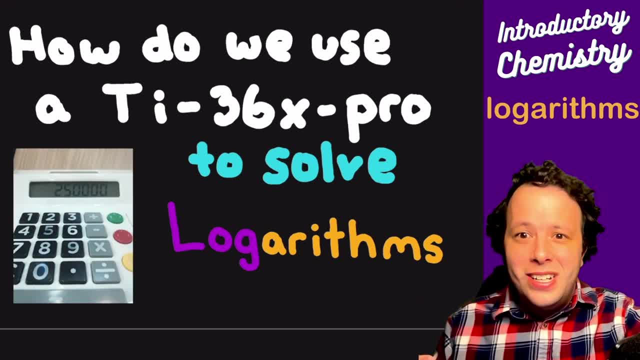 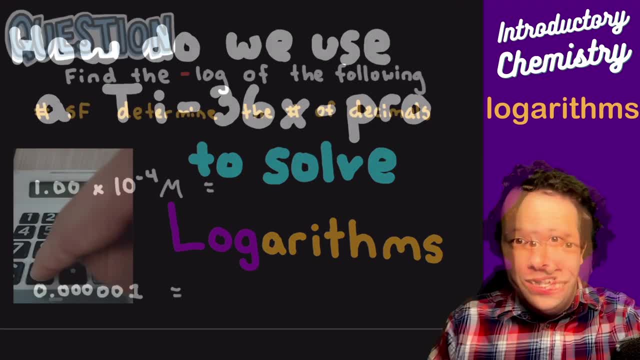 Because you don't want to do all the work and then put the wrong answer on an exam even though you knew how to do it. It's just discouraging and not fun. So let's go forward and take a look at some examples of this. So with our first example, 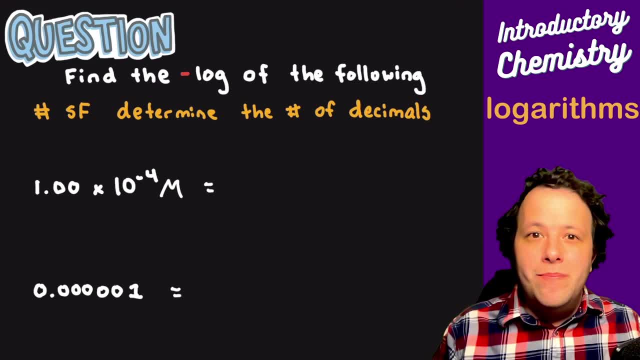 we're going to find the negative log of the following numbers And we're going to also be determining our sig figs. But the first thing is is let's talk about the sig figs. So when we are doing these, sig figs are a little different when it's talking about logs. 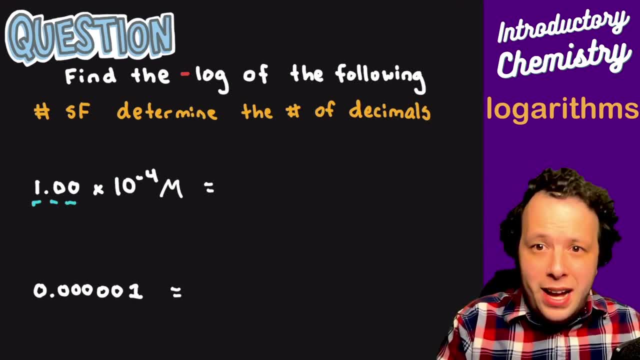 So the whole idea is you count the number of sig figs you have and that's going to represent how many decimal places you have in your pH value. So we have three on the left hand side, so that means you're going to have three decimals on this pH. So if we were to do this- so let's. 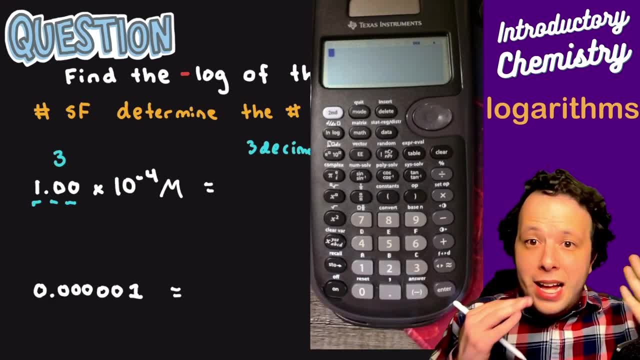 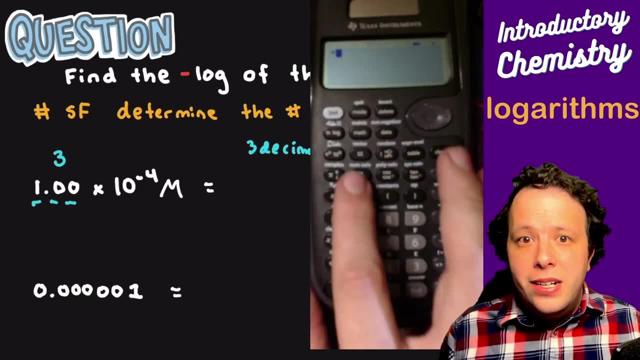 bring up our calculator to solve this. The first thing is is how do we end up using it? So the first thing is is hitting our negative button, So that way we make sure that we do use a negative log. Now the log button is up here on the top left hand side of your calculator, So you can kind of 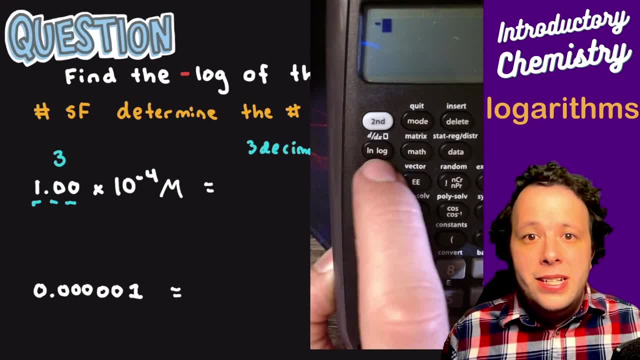 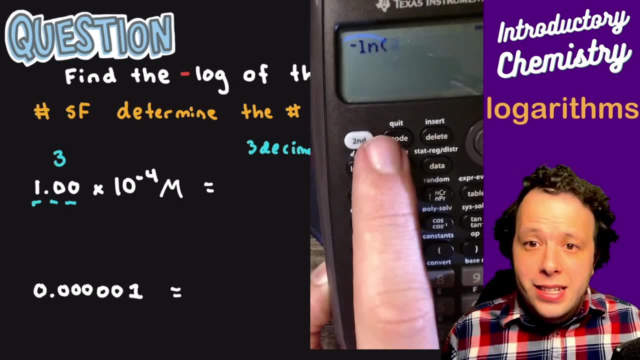 see the log button here, And one thing about it is: you'll notice that there's two different things listed. You have LN and LN. And you'll notice that there's two different things listed. You have LN and LN. So if I hit that one time, that is a log, but it's not the right one. This is wrong. 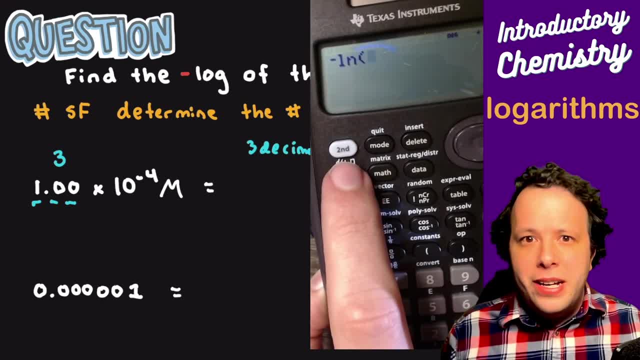 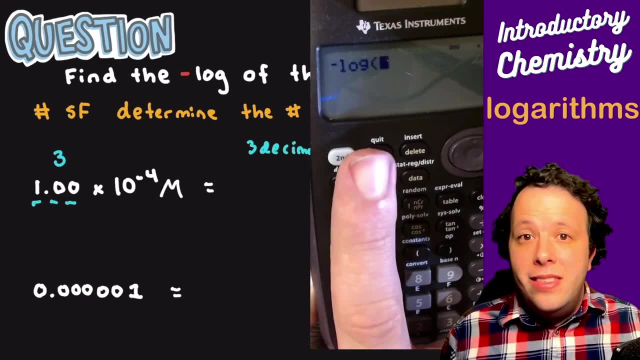 This is a natural log. We use this for different algebra applications and for more advanced chemistry purposes. So what we would do is we got to hit the button one more time and then the log will pop up. So you want to make sure you check Now if you accidentally hit it too many times. 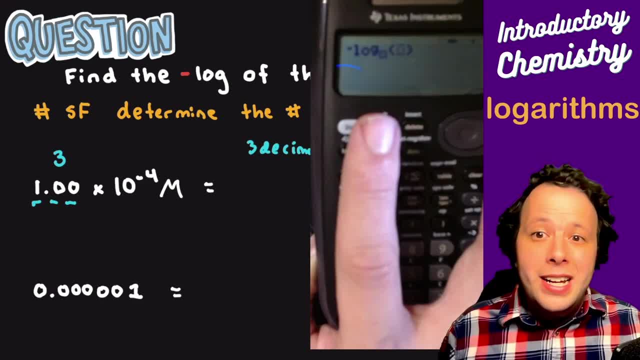 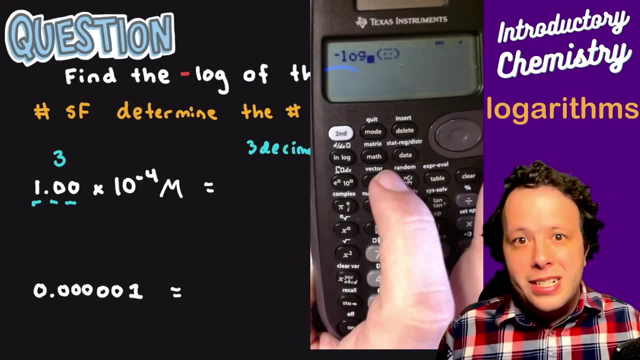 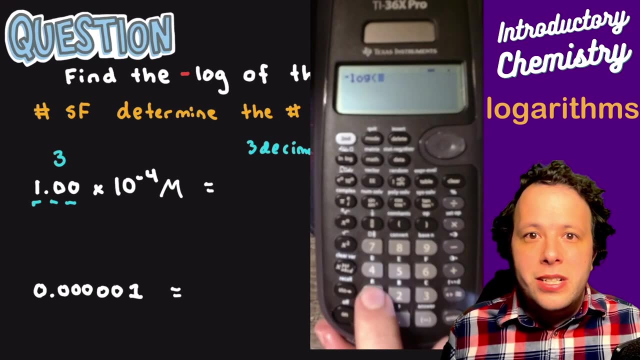 and this pops up. what this allows you to do is you can actually define your base value, which for us is 10.. But the last one that was previously up here was the exact same thing. If you just hit it again, it will pop up the negative log. So now the whole idea is: we're going to plug in our numbers, So we 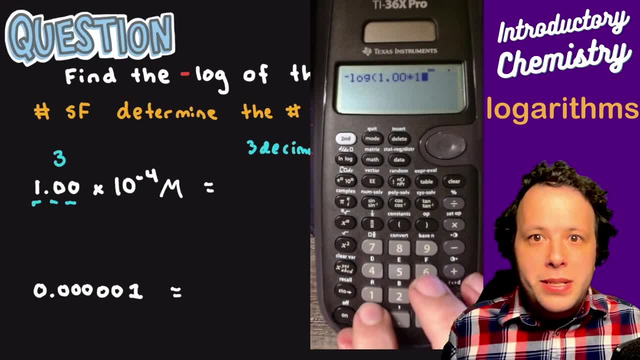 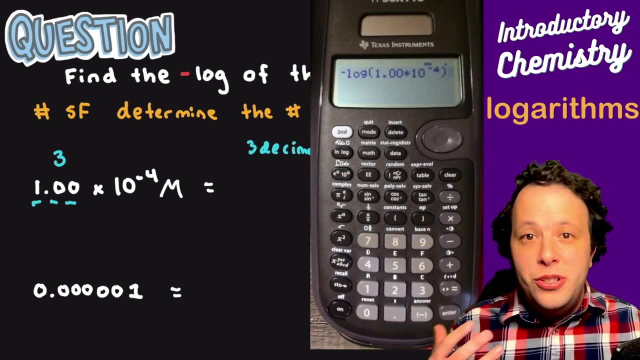 have 1.00, right, And then we would do times 10.. And we're going to raise that, using our power function right here, to the negative fourth. So we hit negative again. hit four. We want to move our cursor over so we can end the parentheses. right, You want to use parentheses as much as you can. 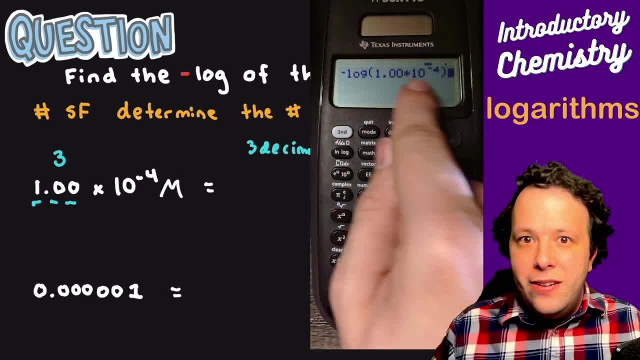 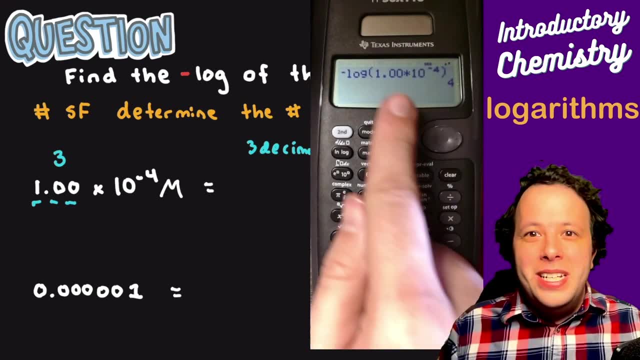 So now we have the following: You want to check We see that everything's plugged in, right? You don't want to blindly start plugging and chugging numbers and not understand them, right? So when we hit equal, we'll get four, which makes sense. It tells you what the power is when this is equal to its. 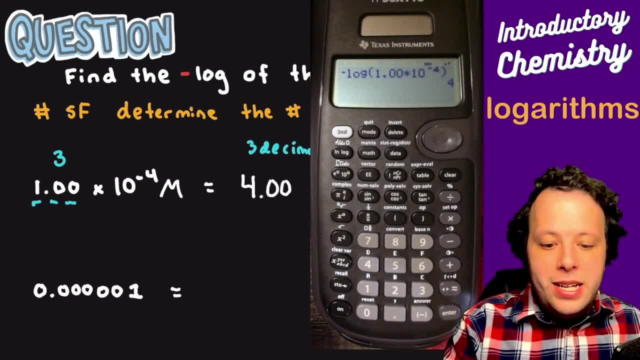 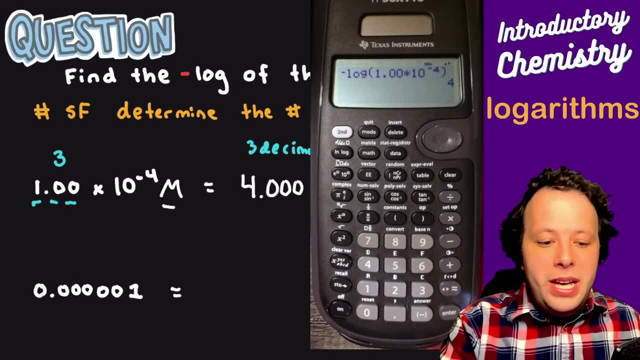 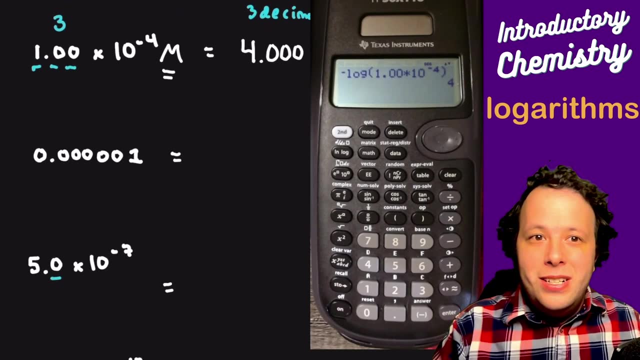 regular value. So we have four and we want three decimals. So it would be 4.0000, which would represent our theoretical pH if we had a concentration of H+. So let's go to the next one. So I have 0.00001.. So if I were to do this, we're going to do the same idea, So we still hit that. 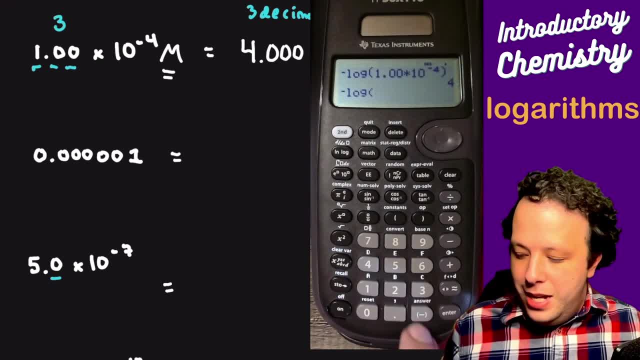 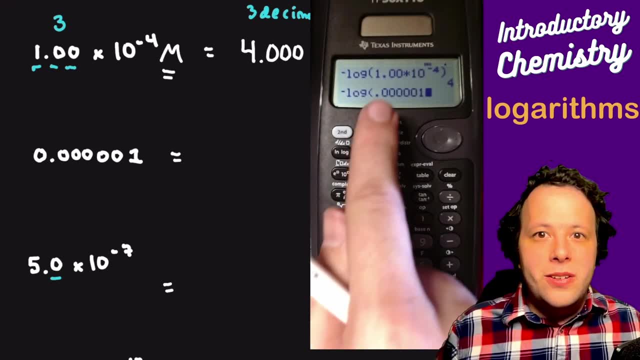 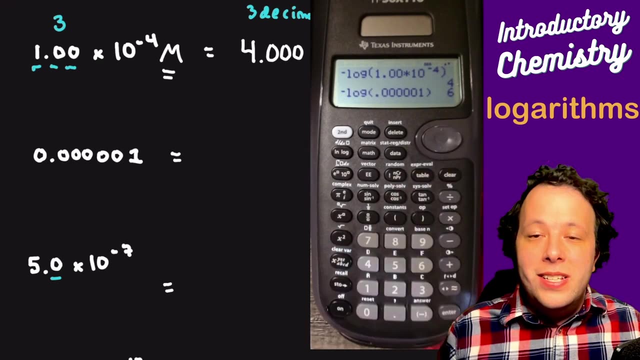 negative log. We'll make sure the LOG pops up And now we will plug in our value. So we need one, two, three, four, five zeros, then one. So we want to just double check that we have everything in parentheses. it equals and we'll have our value. This tells you that that decimal place 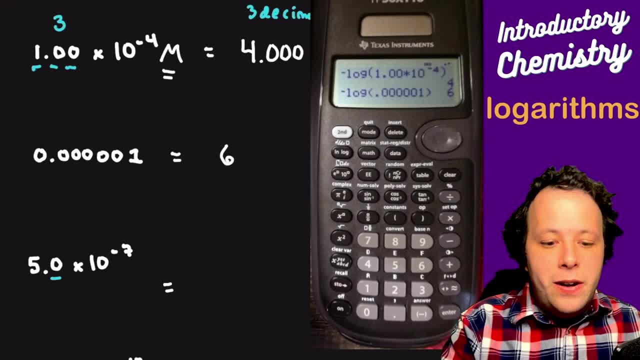 moved over six times, which is what we want to do. So we're going to do that. So we're going to do our pHs, Being that we had a total of one decimal place or, sorry, one sig fig, that means we're. 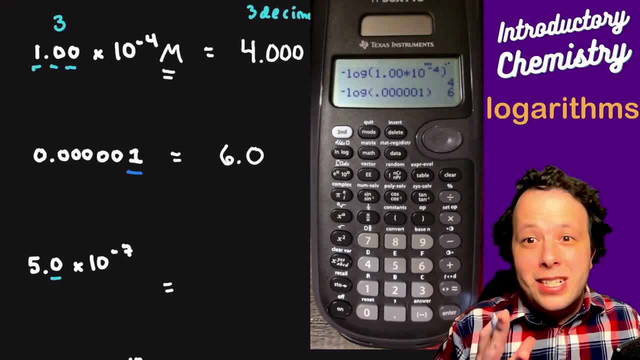 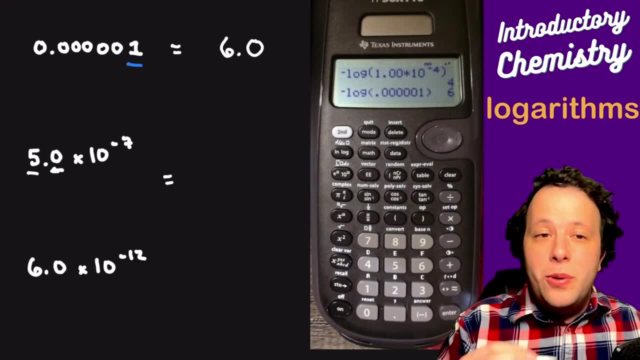 going to have one decimal place with our number, So 6.0.. All right for the next one. one thing we can see here is that we have two sig figs, So that means we'll have two decimal places. So when we do, 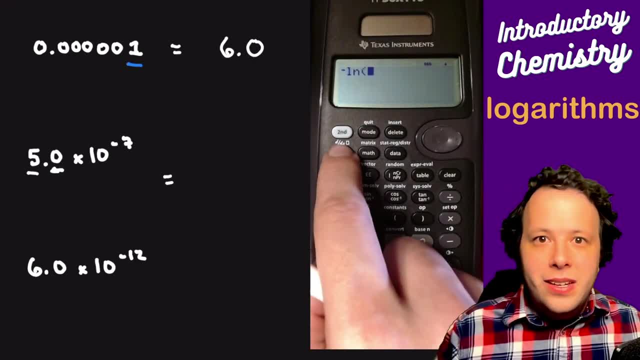 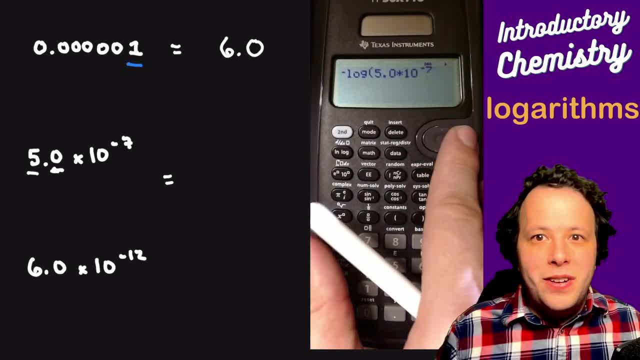 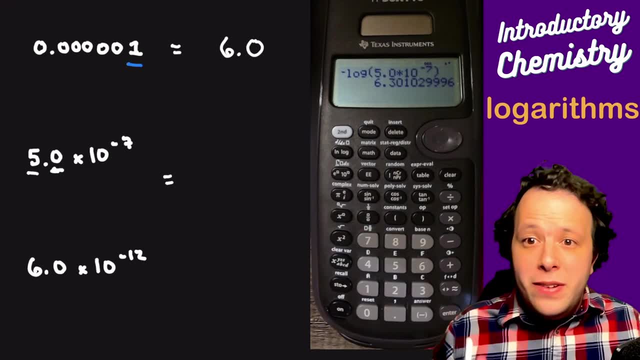 negative seven. make sure everything plugs in, everything looks fine. Now we're going to hit in our parentheses and we'll hit enter. And now this is when it starts to be values that go between pHs. you can have values between, because acidity is a range right. It goes from zero to 14,. 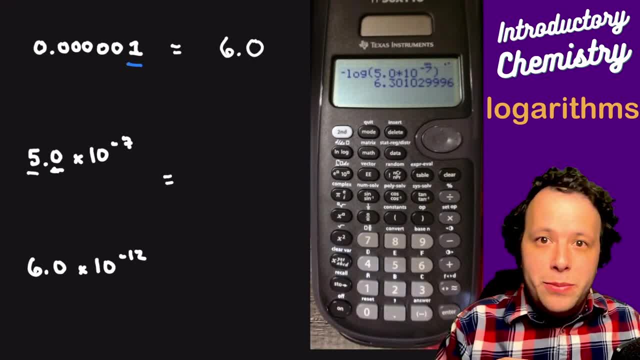 typically So. being that we had two, we're going to want two decimal places, So we'll put six and then we'll put three, zero, and we're going to be rounding here. we see it's next to a one, So we keep it just where it is. 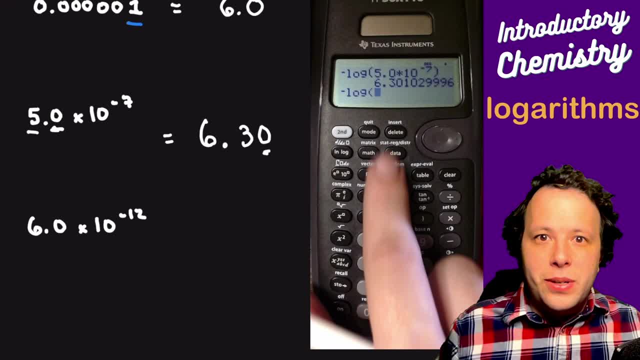 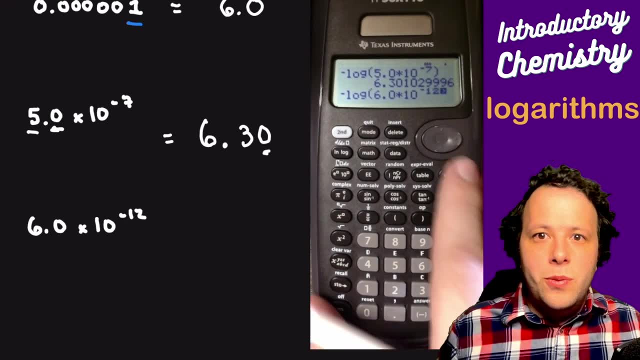 All right, our last one. We have negative log again, So we're going to plug that in Hit 6.0. And we're going to do times 10 to the negative 12.. We're going to end parentheses And now we have our value. 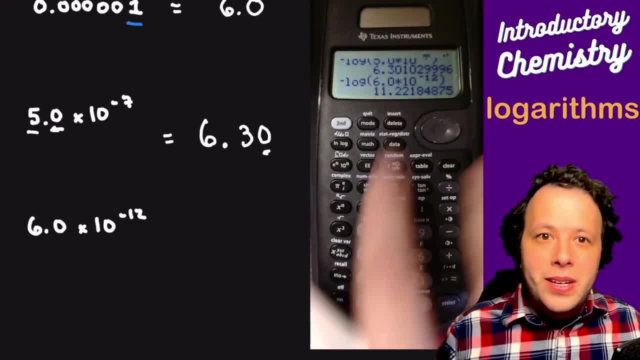 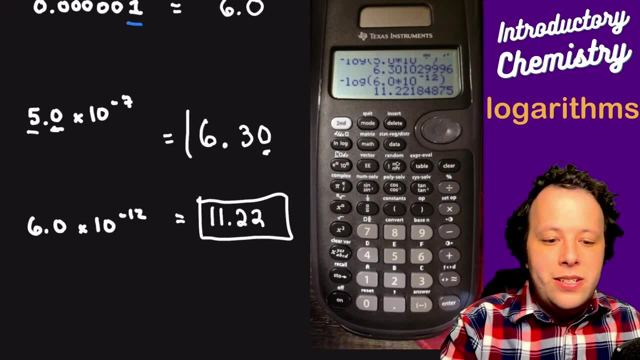 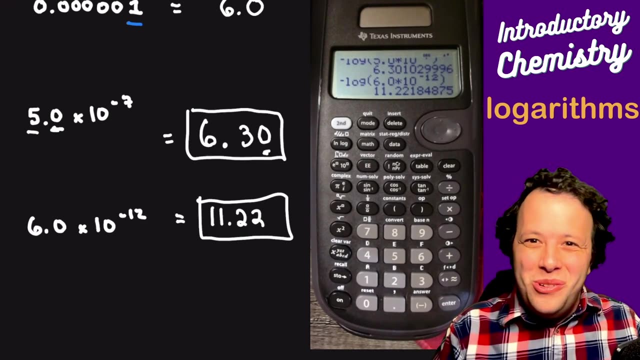 So now, currently we have 11.22.. So we want two decimal places, So we are going to write 11.22 as our answer. Okay, So this is how you go from concentration to pH. Now what about going backwards? Can you do that too? 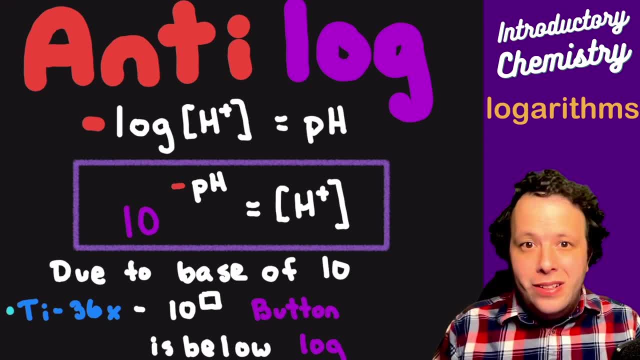 Let's take a look. So, when it comes to canceling a function, this is the same idea as like multiplying versus dividing, Or if you have something that's squared and then you square root it to cancel. Well, in terms of logs, 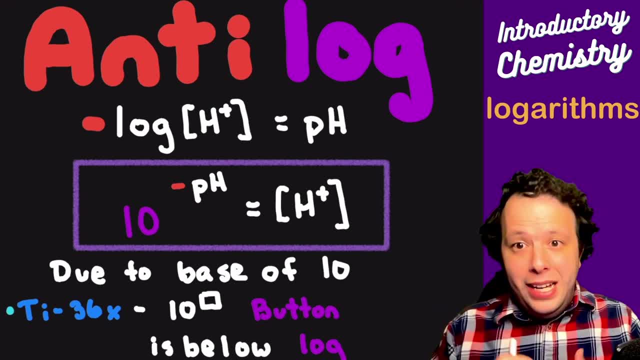 we have an anti-log in order to cancel it. Now the anti-log is using the base, So whatever value that is Now being for us, we're assuming that this is a as 10 to a power right, So whenever we have negative log. 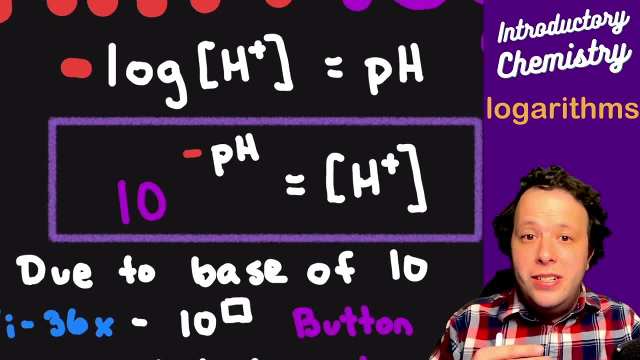 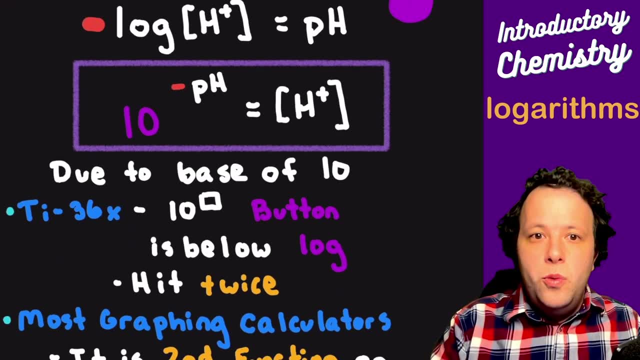 we just use 10 to the negative pH to cancel that out. Now, how exactly do we use that with our calculator? Well, that's a lot a little bit simpler to use. So, when it comes to your TI 36, so the calculator we're using here, 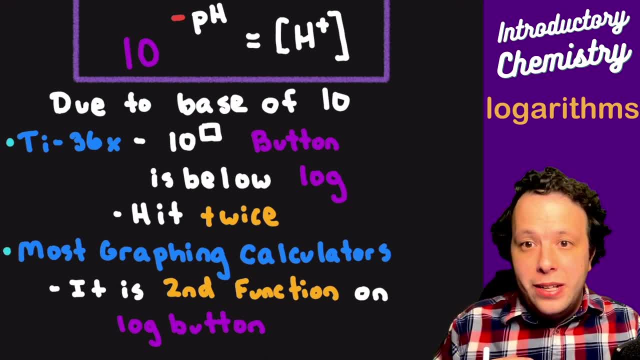 you have a couple of different options for how to cancel out your values, And I'll show both of them. There is a button that's designed for this, And I don't think that the creators of this calculator really put it in the best location. 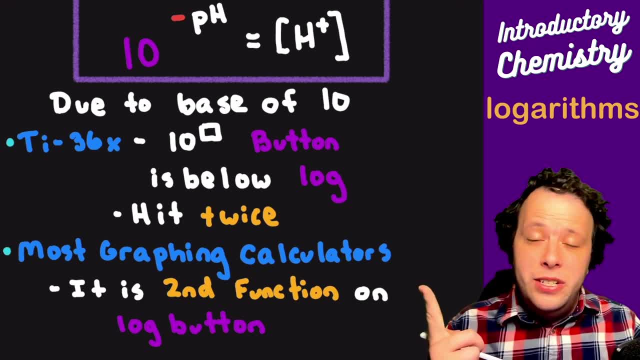 It's close, but it's not how, like the graphing calculators do, Many of those will actually show. it will be: You'll have a second button on your calculator and it's generally the function that's. the second button is how you can cancel out all the functions on your calculator. 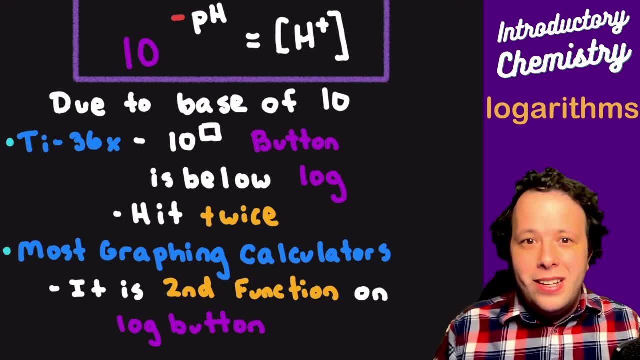 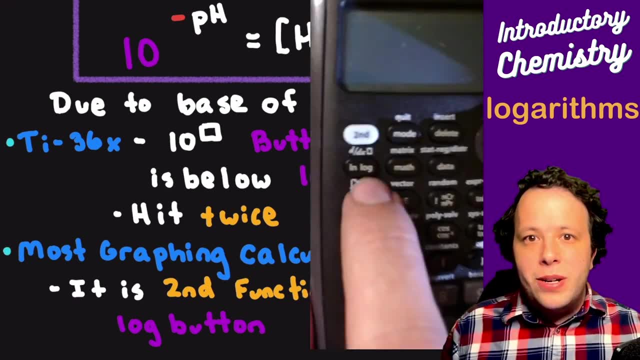 It's actually really nice. So let's take a look at exactly where that is and how we'll do that. So if I put my calculator back on right now, so if we see the log button which is right here on the top, 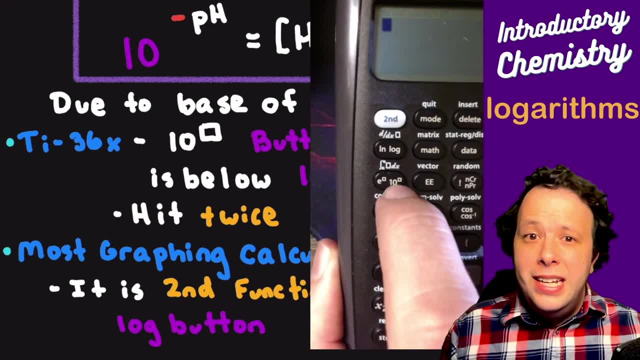 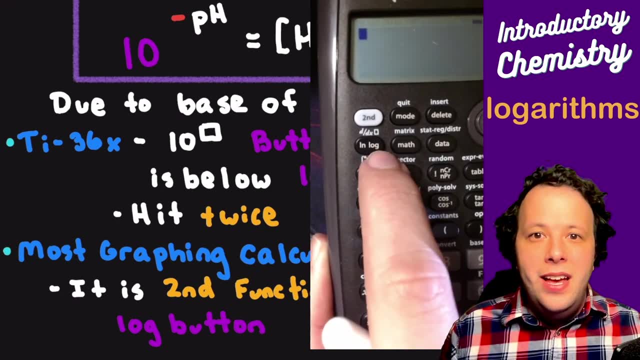 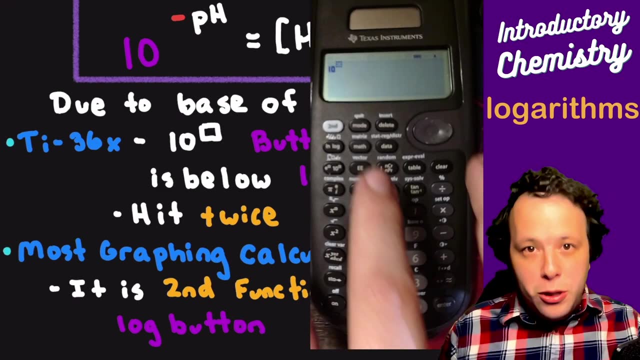 So You'll see right below it is that here is this E button and then the power 10.. These are the opposites of natural log, which is the E function, and then 10 to the power. So you could just hit this button twice to get 10 to the power of your pH. 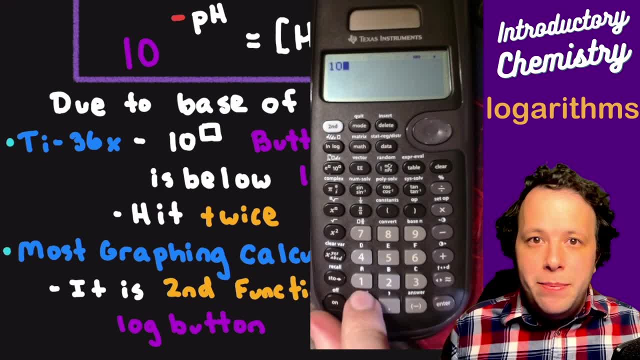 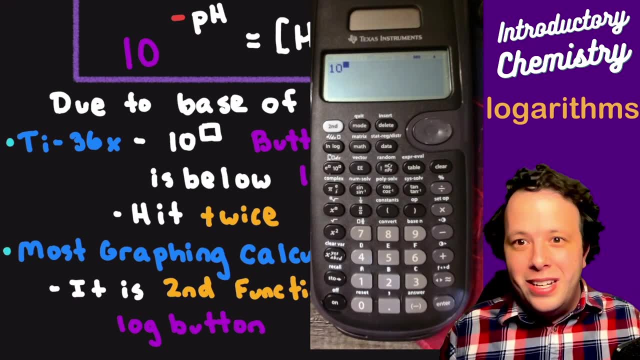 Now the other way you can do it is you could simply just type in 10 and then put your power button and then plug it in this way as well. That's usually the easier way, because probably 99% of students are used to. 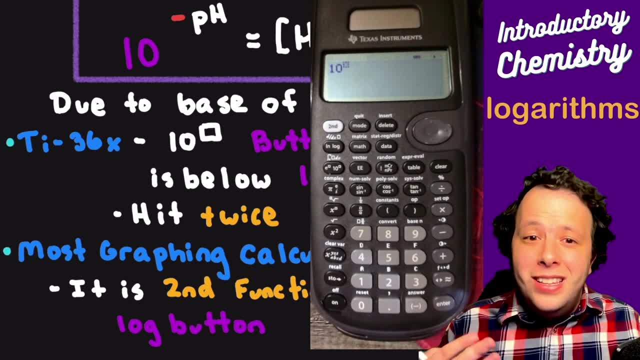 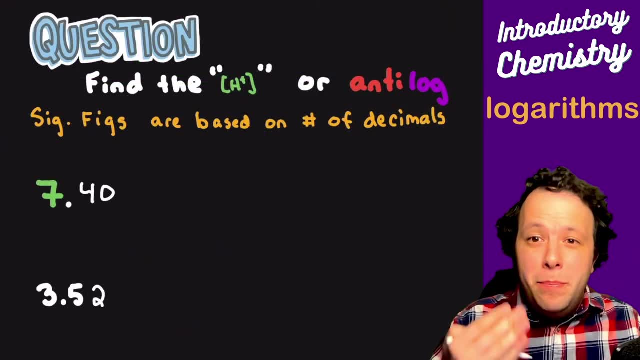 Using that already when it comes to their functions. Let's do a couple of examples together and then we'll be on our way. So let's find our theoretical H plus concentration based on our, on our pH values. So we're going to use the antilog to do that. 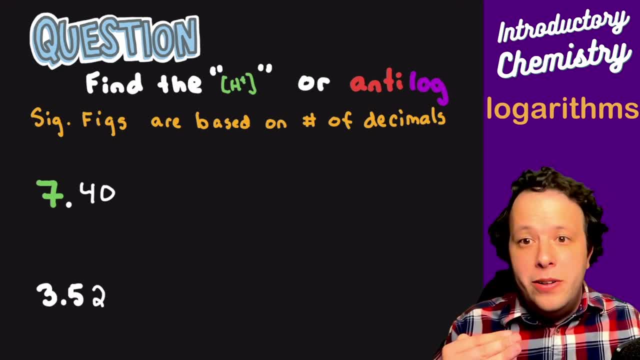 So the thing here is the sig figs are based on a number of decimal places you have. So, like on the first example, right, we have two decimals, So that means that your concentration is going to be two sig figs as well when we calculate that. 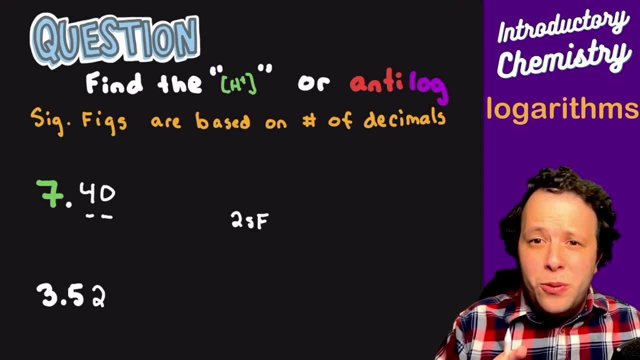 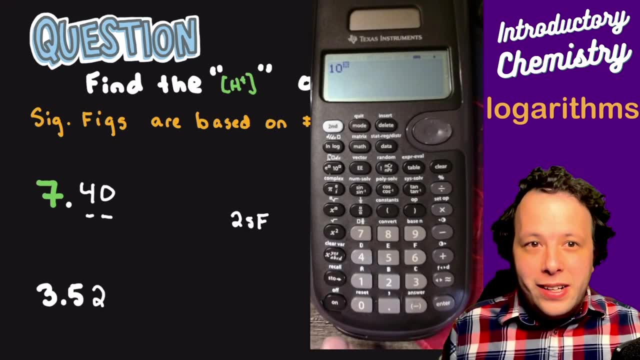 So sig figs- Figs are always important, especially if you have to record them digitally- and a lot of your homeworks and labs. So let's take a look, Let's use our calculator to actually do this. So if I bring up my calculator so before, I still have the ten function here. 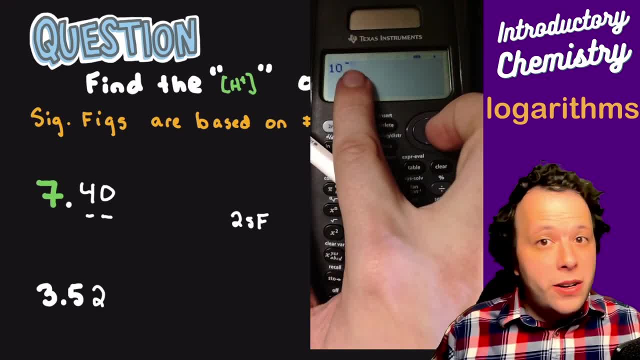 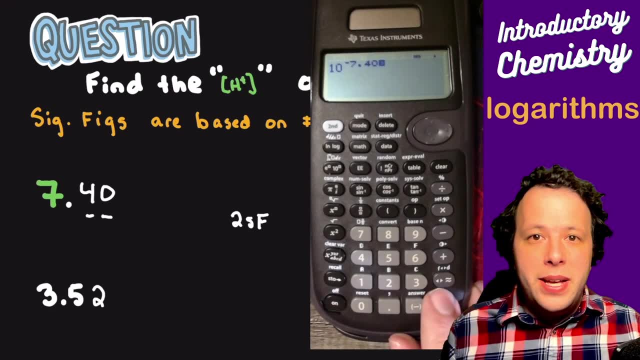 what I'm going to do is I'm going to hit the negative sign. So that's really important. Are you going to get a value that doesn't make any sense? Then we'll put seven point four, zero, So put that whole value in, and then also we have to hit equals. 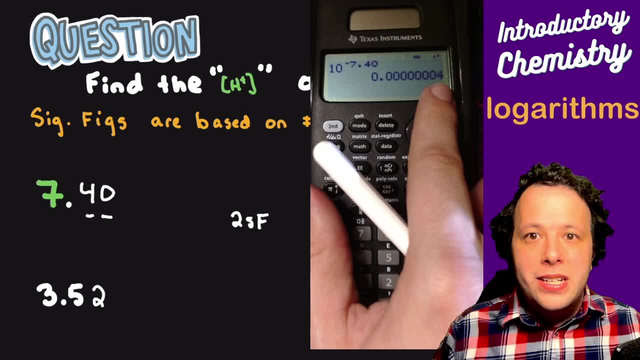 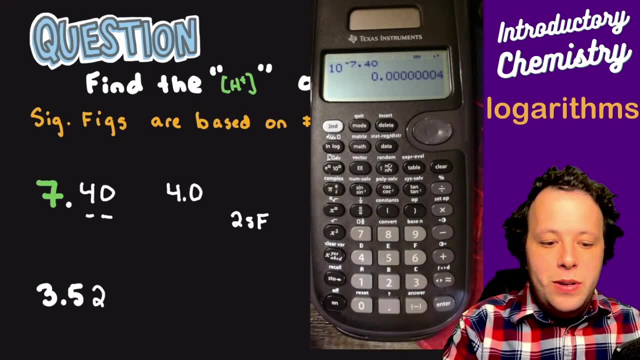 And now, what this shows you is how small your value is. So what we have is our four value, And being that's going to be four point zero, then we just got to move that to a power which we got to count. how many spots does this move? 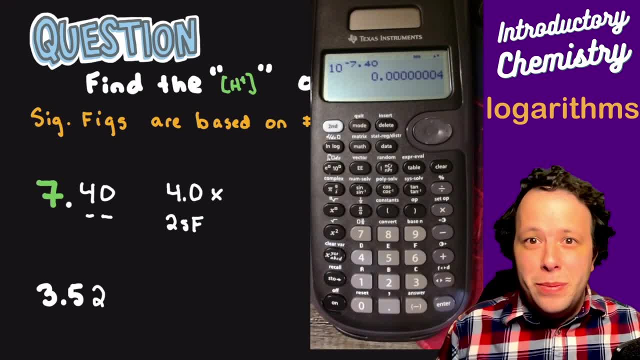 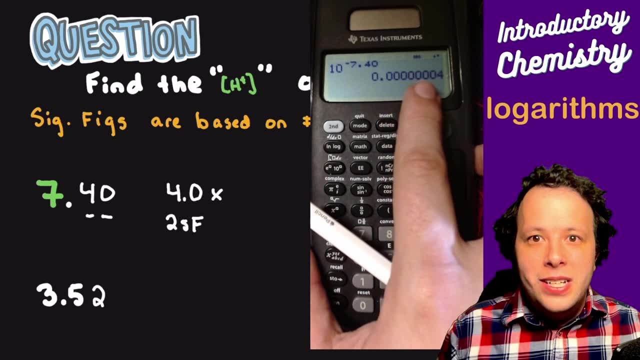 Now, if you're lucky, maybe your calculator has how many spots that's going to move. But for me I always go the old fashioned way, So we're going to count. So we have one, two, three, four, five, six, seven, eight spots. 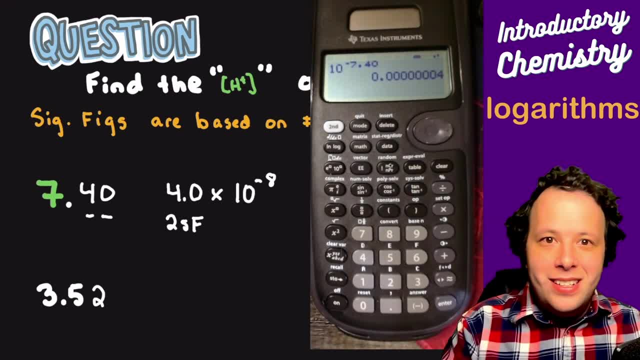 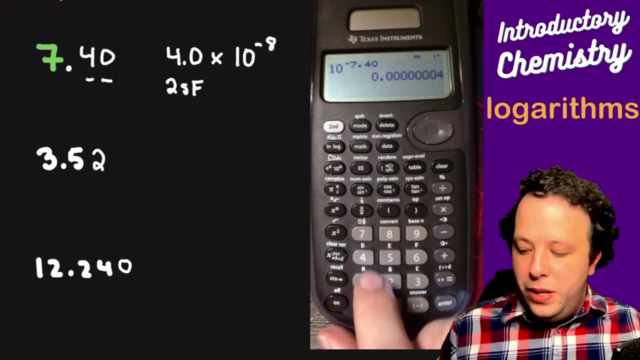 So we have four point zero times ten to the negative eight, Their first value. Let's go into another, So the next one. we have Three point two. So what we are going to do is I'll show you how to use the other way. 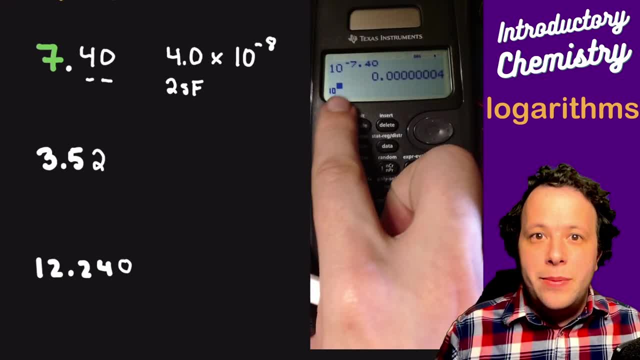 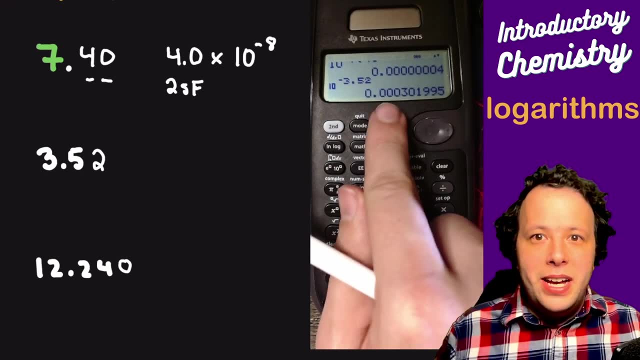 So we're going to do the ten button, So we're going to hit that twice to make sure it says ten. And now what we'll do is: we'll raise that to three point five, two, We'll hit equal. And now we have our new number here. 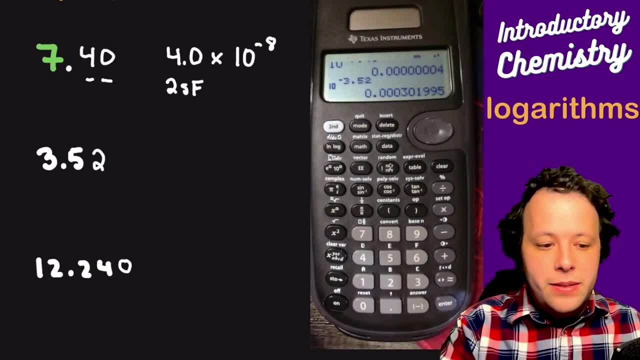 So, being that we had two decimal places, we need two sig figs. So we are going to say three point zero times ten And we need to count how many spots. So we have that that's four positions. that moves. There's going to be three point zero. 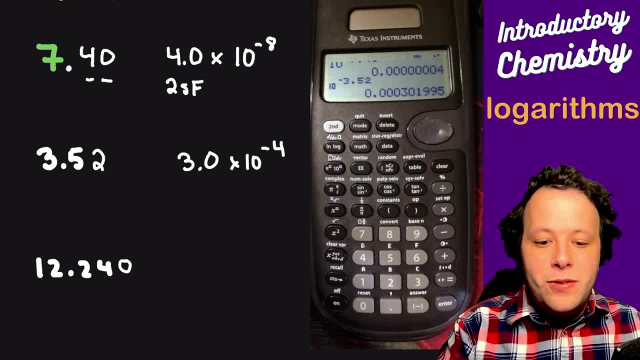 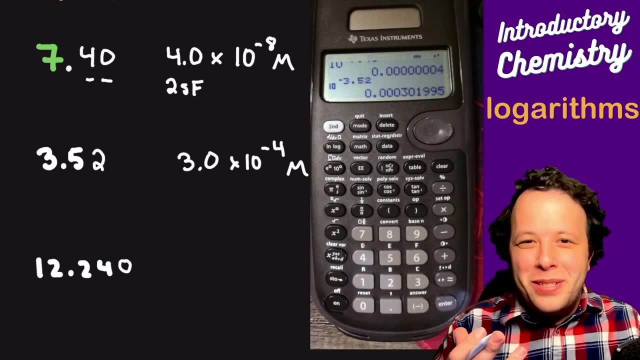 Times ten to the negative four. And remember this represents, these represent Malarities, is what these shows. So remember units. your professors expect it now for the next part. right, So one more. So if I do the next one, we would. 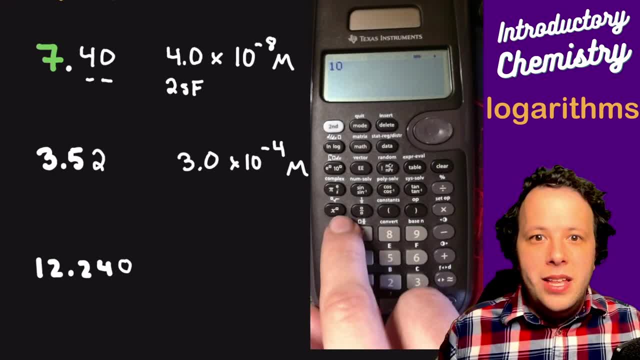 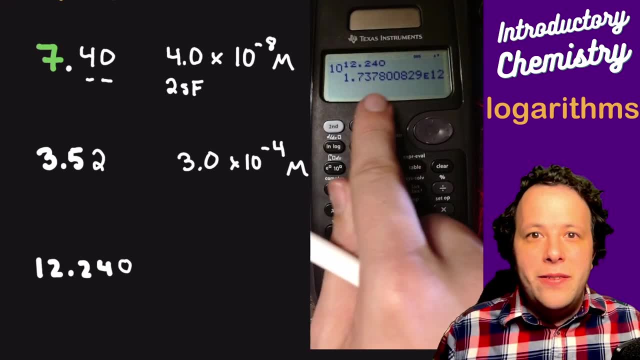 So let's clear our work. And now we have ten, and we're going to raise that to the power, And we're going to say twelve point two, four, zero, We'll hit equals. And now we have a very, very big number. 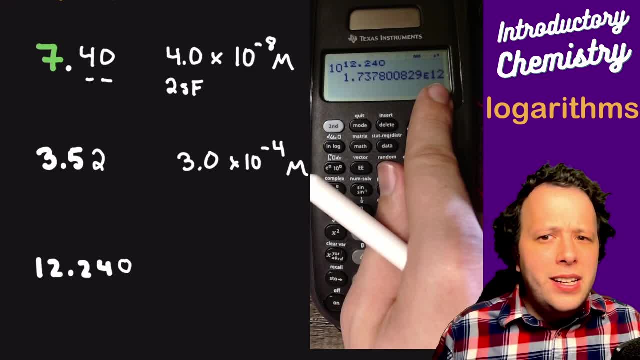 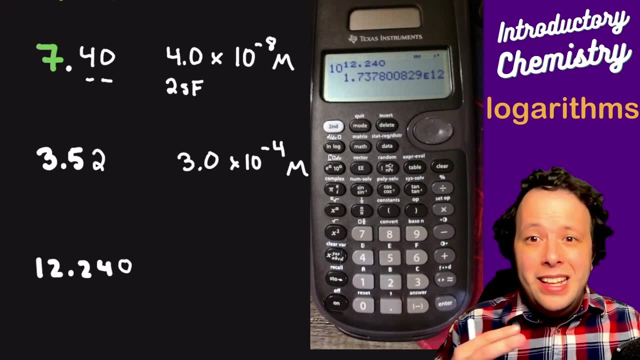 Now, why is it so large? Have I forgotten anything while doing this? Notice, I forgot my negative sign. right, These should be small concentrations. They shouldn't be anything that's massive. right Ten to the 12th: Malarity isn't feasible. 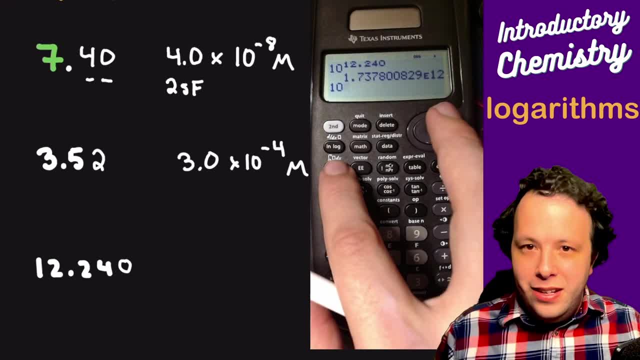 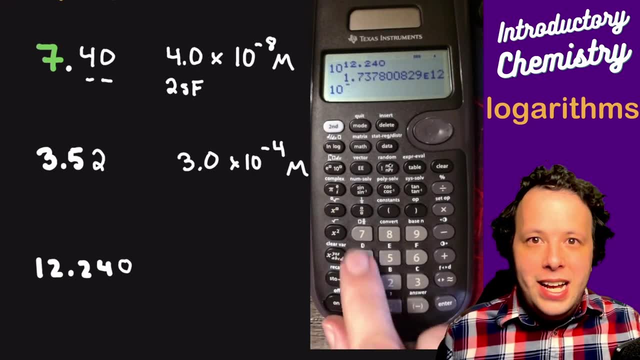 So let's fix that. So what we'll do is I'll hit my ten again, I'll raise that to essentially the power in order to fix that. So let's do that. And now we got to hit our negative twelve point two, four zero. 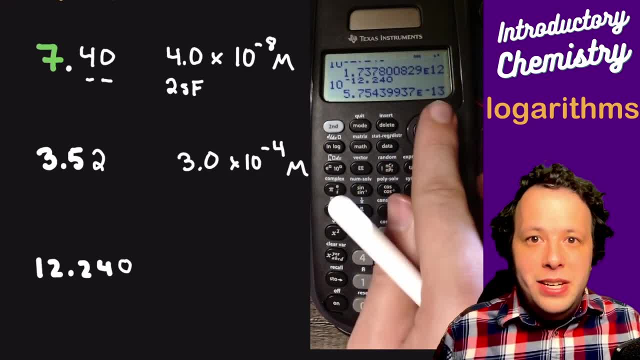 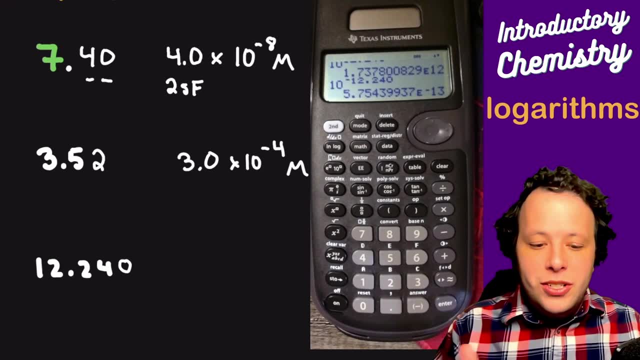 OK, so now when I change that, we kind of see how different the values are: Right Almost ten to the 12th, This one's ten to the negative 13th. It's supposed to be tiny, So especially when you have a high pH it should be very small. 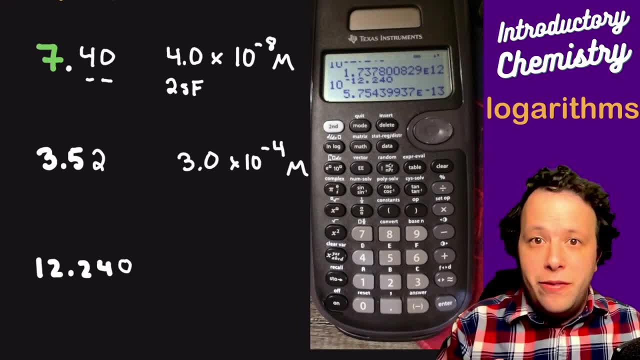 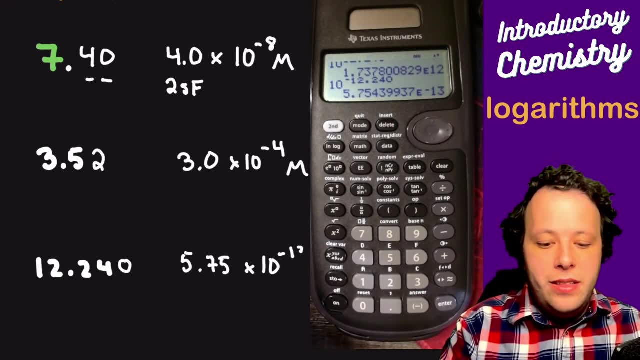 So when we do this right, we have three decimal places, so we'll have three sig figs. So we're going to have five point seven five, Then we're going to ten, to the negative 13.. Malarity will be our answer.